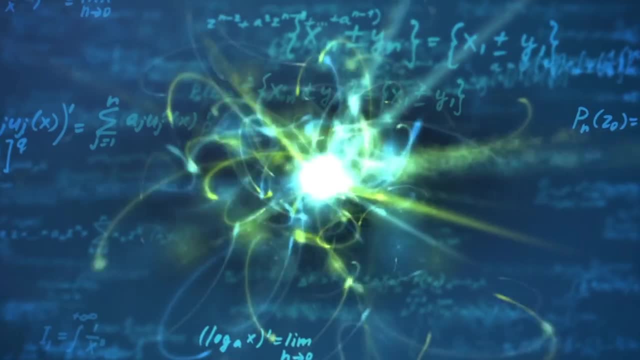 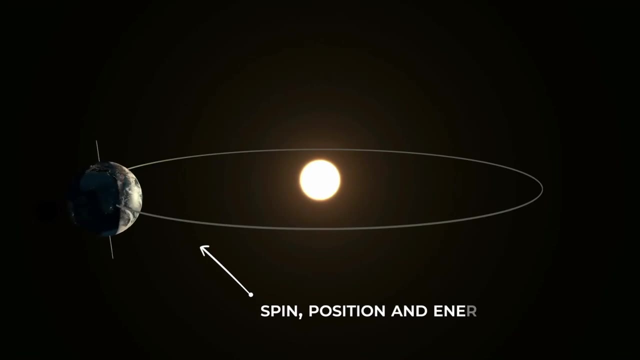 Why are we stuck in it? What if we don't get to know? what is so crazy about quantum science? The Weirdness of Quantum Superposition. Early quantum research found that quantum particles have measurable properties called quantum states. Some examples of a particle's quantum state are its spin position and its 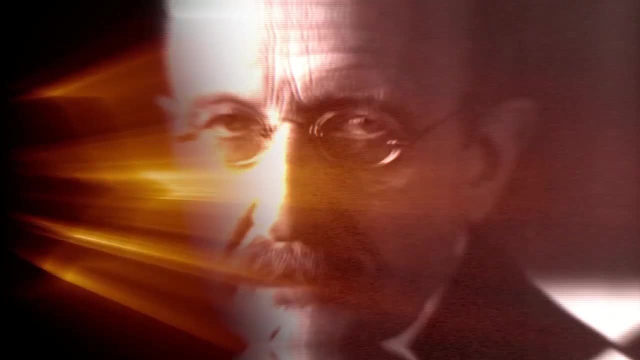 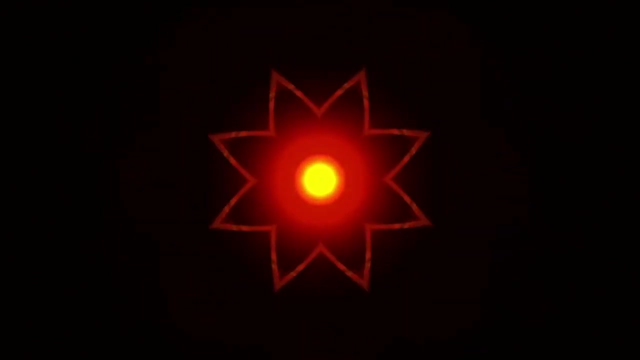 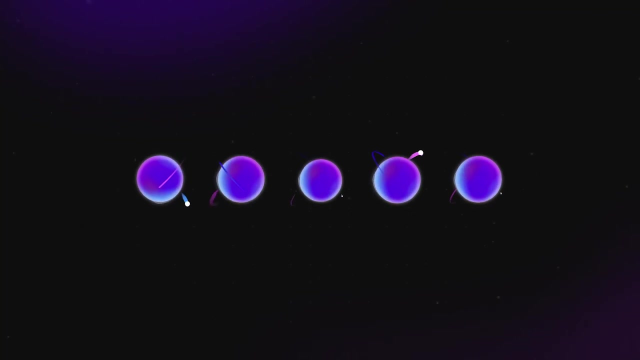 energy. Scientists were able to discover that in certain scenarios, these subatomic particles have an interesting feature that allows them to occupy multiple quantum states at one time. This ability to be in multiple states at once is called quantum superposition. The concept of quantum superposition wasn't discovered until the mid-1930s by the famous 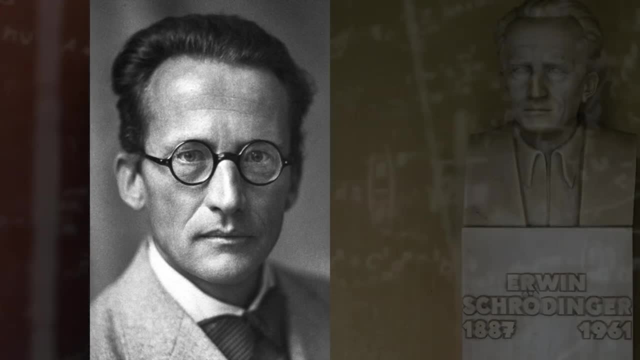 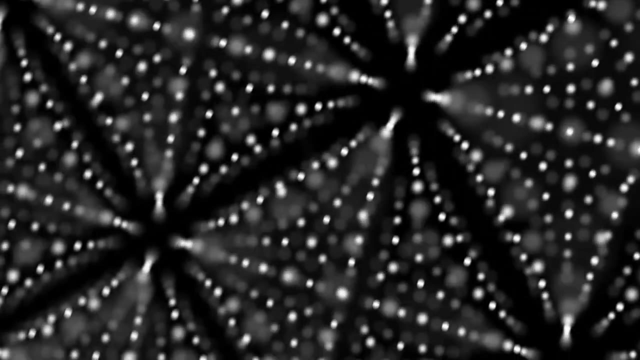 physicist Erwin Schrödinger, who is now known to be one of the founding fathers of quantum mechanics. But quantum superposition seems impossible, doesn't it? How can this be possible? How can a particle have multiple values for a state? 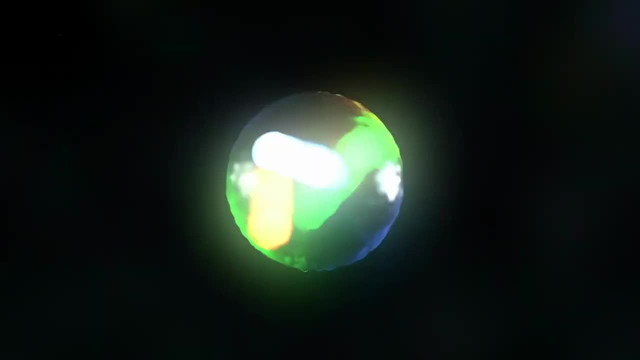 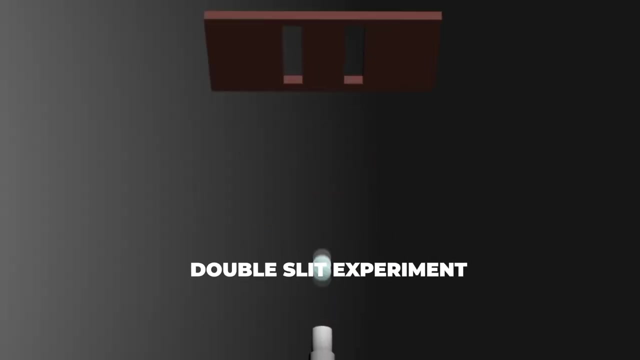 Well, the world of quantum mechanics is ripe with these types of phenomena that defy the conventional logic that we're familiar with. One popular example of quantum superposition came in the form of the infamous double-slit experiment, which has been repeated again and again with the same result. 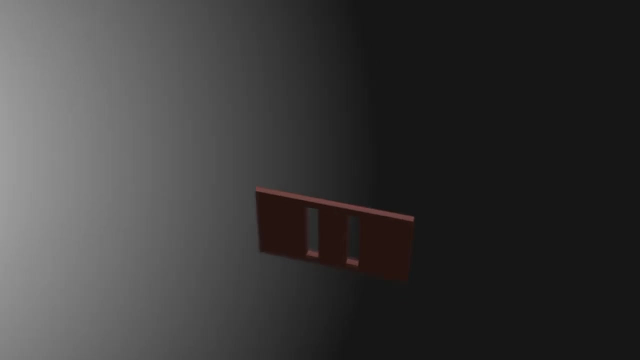 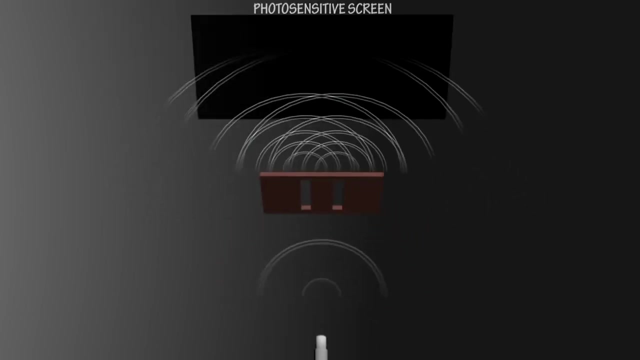 Although it was first documented in the early 1800s that a beam of photons- little bits of matter incident on a screen with two slits cut out will create an interference pattern when measured on the opposite side of the screen. The double-slit experiment showed that photons 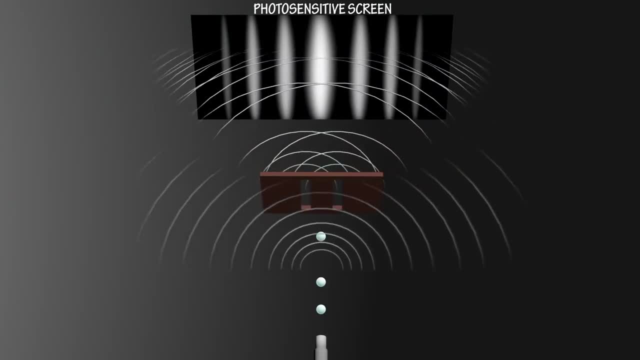 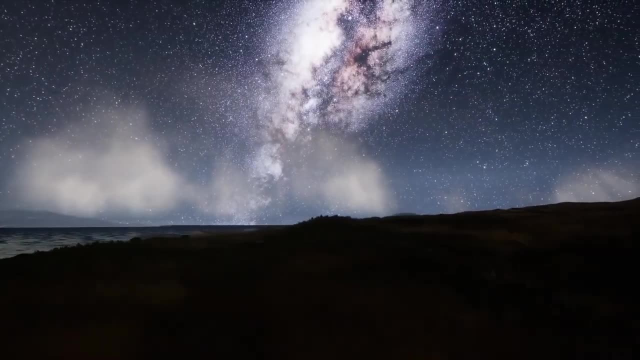 will interact with each other and form an interference pattern identical to that of a wave. The reasoning that the photons were simply bouncing off each other held up for over a century and a half. But the final bit of weirdness in the double-slit experiment wasn't found until 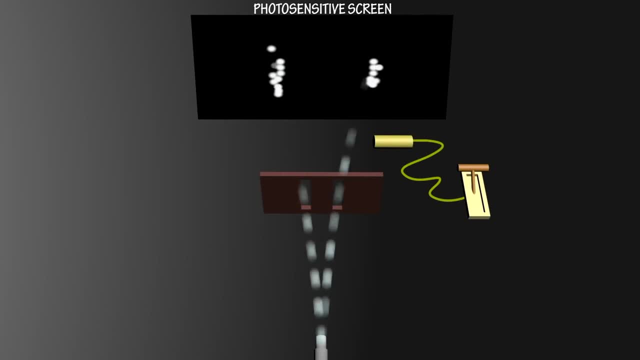 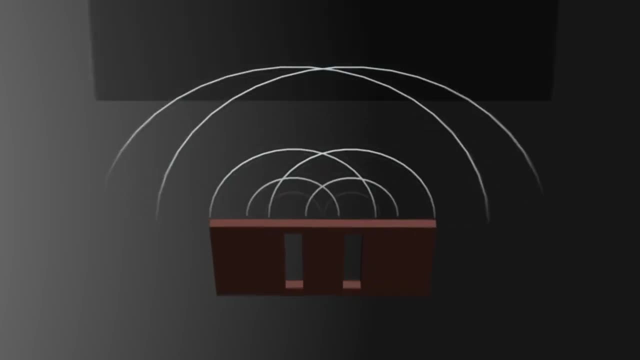 1971, when the technology existed to fire photons at the slits one at a time. What they found was that, after firing these single photons through the slits for a long time, the same interference pattern from firing a beam of photons appeared. 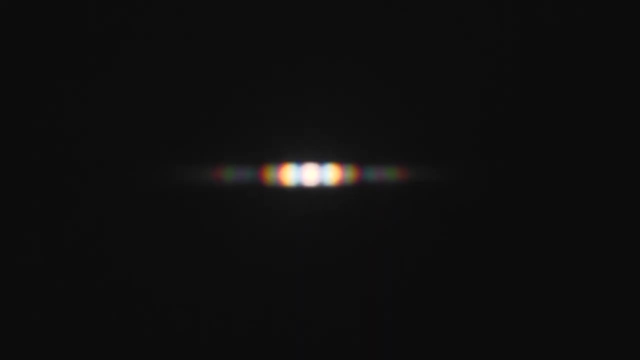 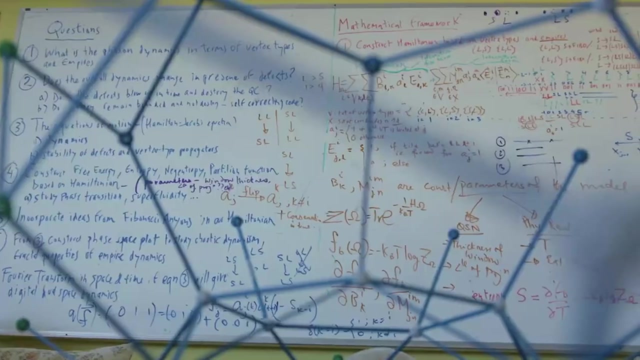 The only conclusion that scientists could come up with was that the singular photon traveled through both slits and interfered with itself on the other side. Regardless of how scientists felt about this, it was clear that subatomic particles can exist in multiple places at once and were able to develop complex mathematics that can explain these bizarre interactions. 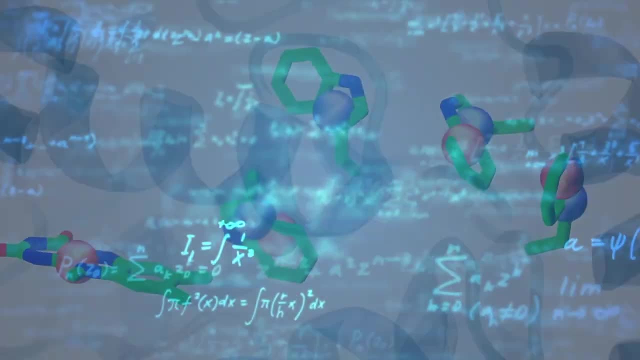 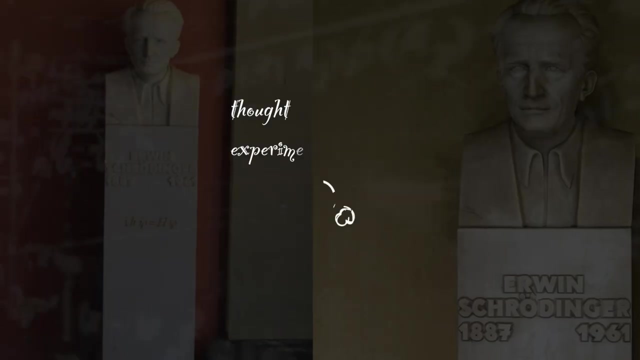 While this whole concept of quantum superposition makes sense in the math of quantum mechanics, it can be hard to explain much of this realm's strangeness using just words, But Schrödinger was extremely smart and came up with a brilliant idea. 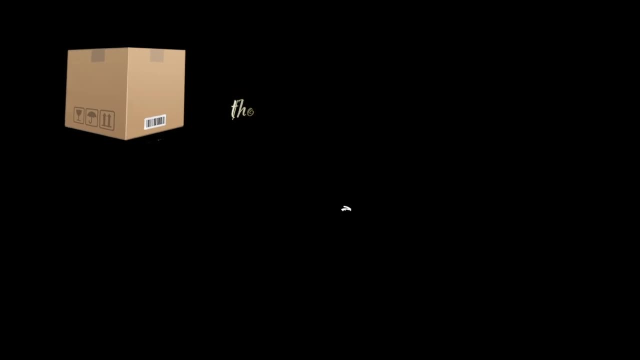 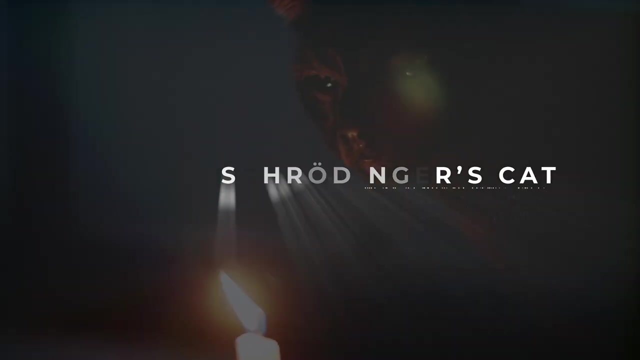 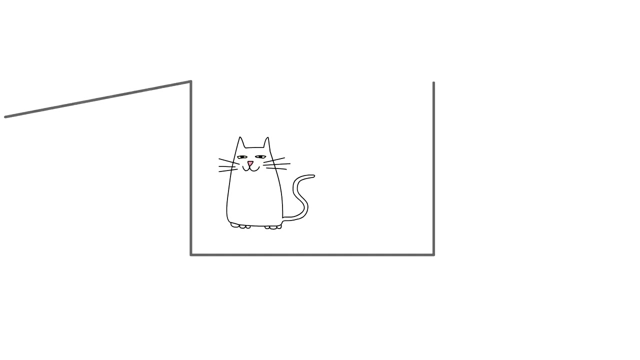 He developed a brilliant thought experiment to help people understand this phenomenon, involving a closed box, a cat and a radioactive material that may or may not decay. Schrödinger's Cat. In Schrödinger's thought experiment, we're asked to picture a cat being placed inside of a closed box with a special contraption. 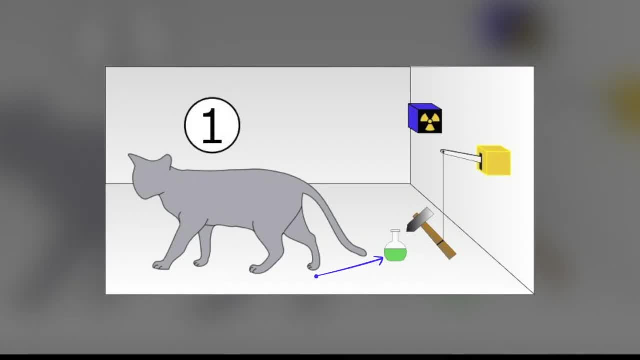 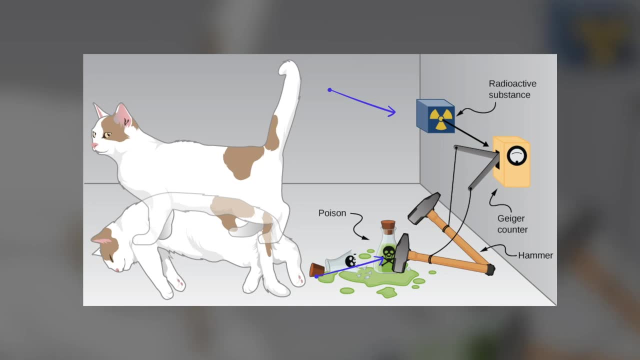 This contraption was made of a bottle of a toxic substance and a hammer attached to a Geiger counter that contains a small amount of radioactive material. The material has a chance to decay, which will then set off the Geiger counter and release the hammer, shattering the toxin. 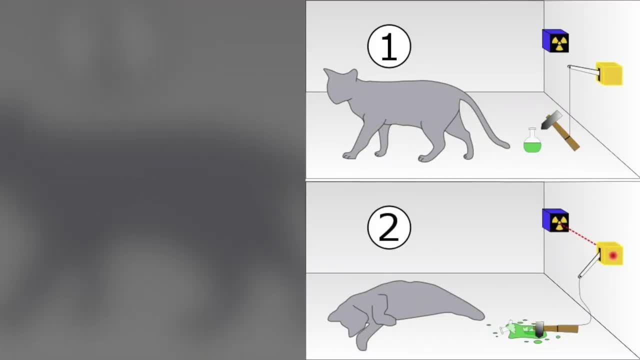 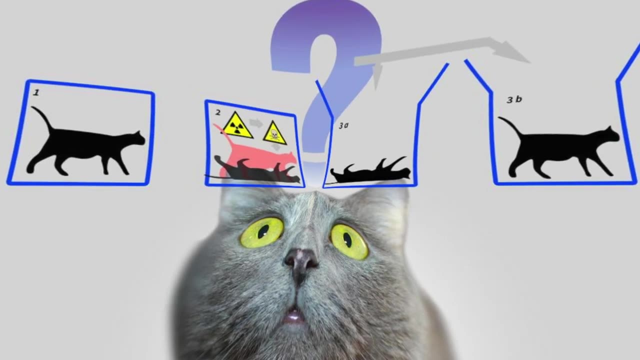 But there is an equal opportunity that the radioactive material will not decay and thus the hammer will not smash the bottle, Because there is an equal chance that either scenario will occur in a given time. before the box is opened, the cat exists in two. 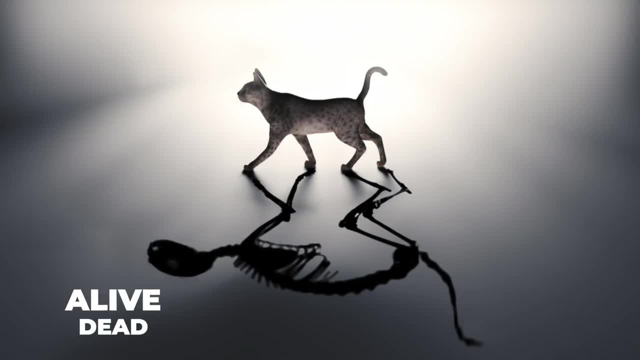 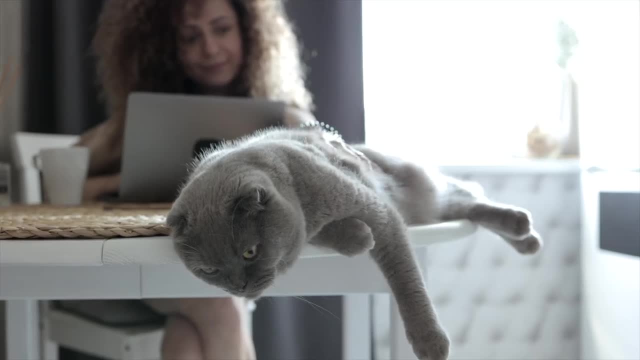 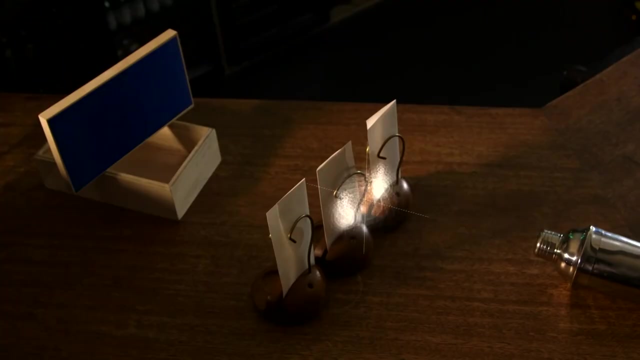 equally likely scenarios, that of being alive and dead with no way of knowing unless we open the box. Only opening the box and looking inside destroys this closed system and forces the cat back into only one state, Much like the results of the double slit experiment, the cat existed in two separate states until an outside observer 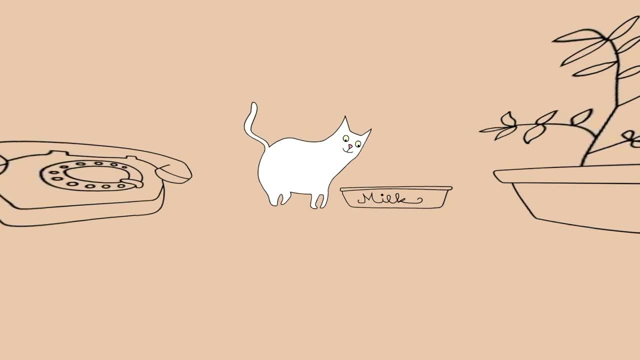 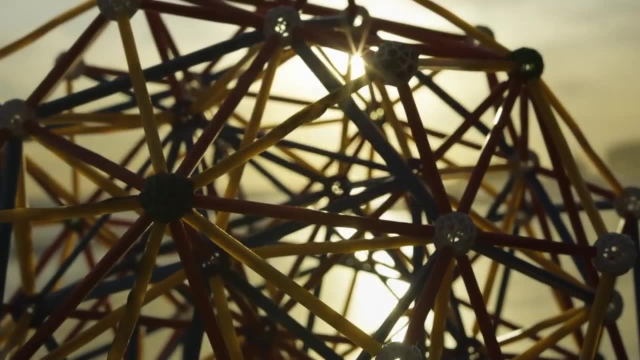 took a look into the system, added energy and caused it to exist in only one state. While the evidence proving quantum superposition as a part of reality was met with mixed enthusiasm, some scientists were jumping at the chance to be the first to find a practical use for this new discovery. 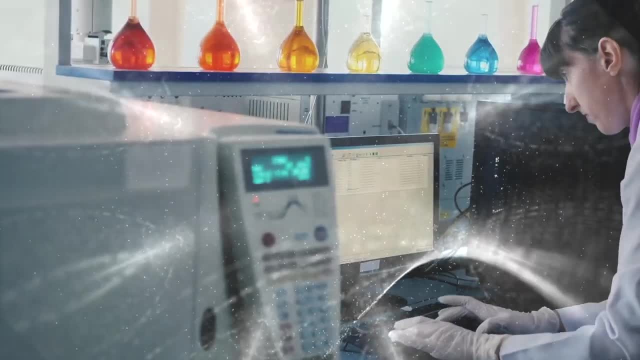 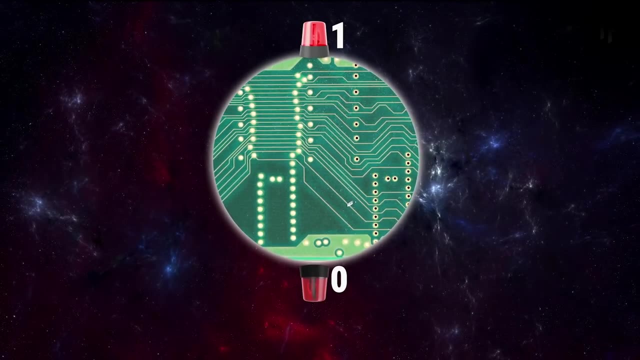 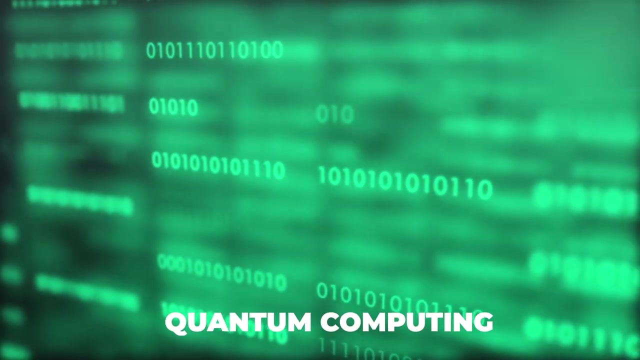 What applications could take place. Let's take advantage of this mysterious feature of subatomic particles. Applications for quantum superposition. One application of superposition that has shown a lot of promise in the past few years has been in the field of quantum computing, Where traditional computers use a binary system that only has two possible states. 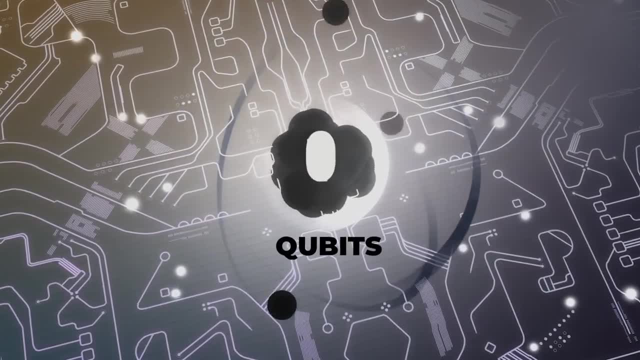 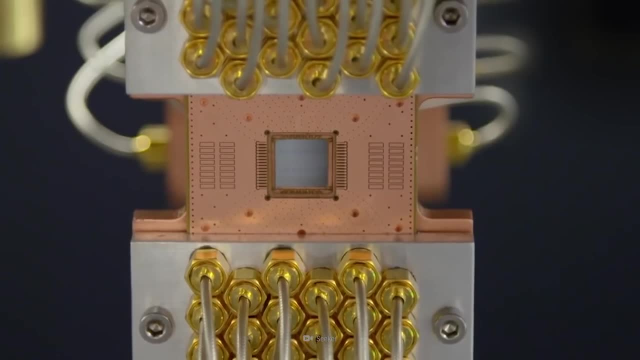 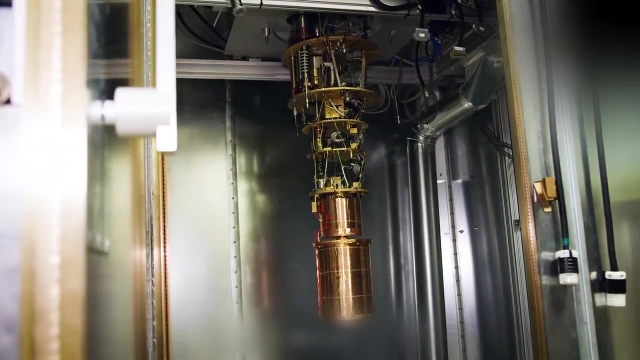 quantum computers use something called qubits, which can be in many different states at once. This allows a quantum computer to work with much more information all at once and allows for much more and much faster processing. Scientists have been motivated by the number of possibilities available with superpowered quantum computers that seem to be endless.